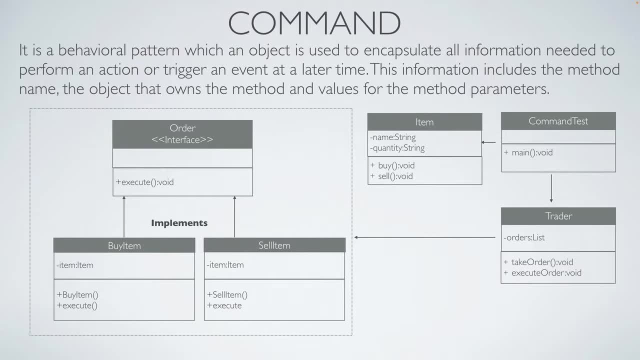 In this a request is wrapped under an object as command and passed to the invoker object. The invoker object looks for the appropriate object which can handle this command and passes that command to the corresponding object which executes the command. Let's take an example of a trader and an order. Let's say a trader can buy items and sell those items. So sell items and buy items could be different kinds of commands. 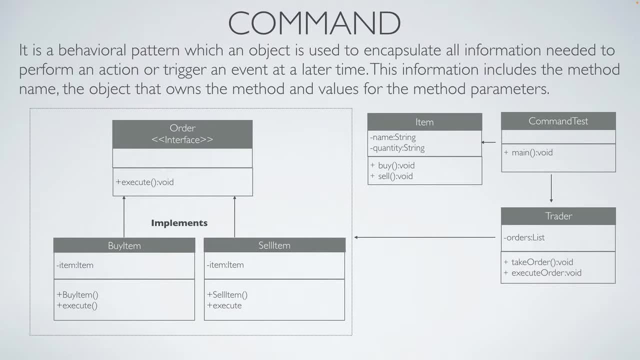 The trader will have methods like take order and execute order, Based on the type of the order that needs to be performed. it would be passed to the corresponding object, The trader will have all the required data and it would be passed to the corresponding commands to be executed. 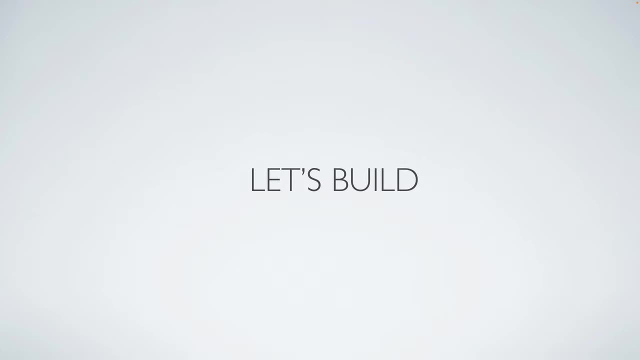 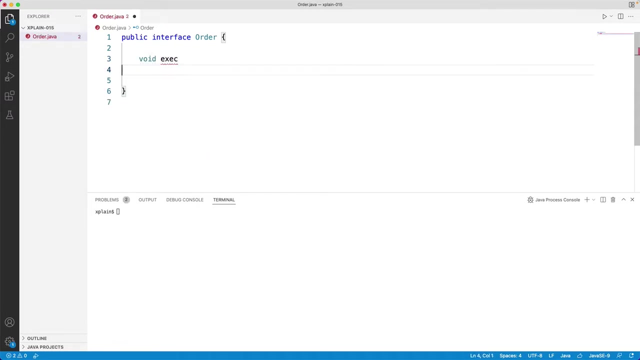 Let's build this example and see how it works. Let's open our Visual Studio Code And here we create a new file called order. New file: orderjava. This is an interface that will have void execute method, And the next one would be: 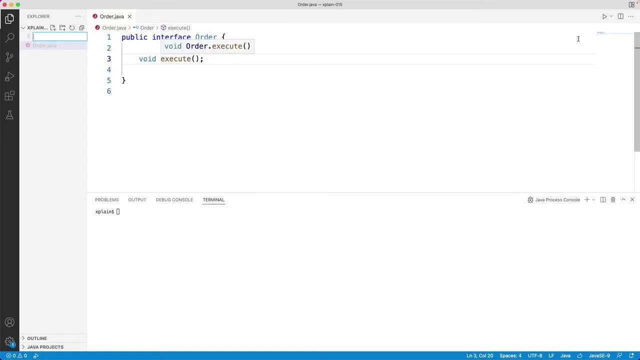 Item Item that we need to trade, So we will call this as itemjava. Within this item we will have the item name, That is public string name, And let's take this name as apple, And the next attribute would be: 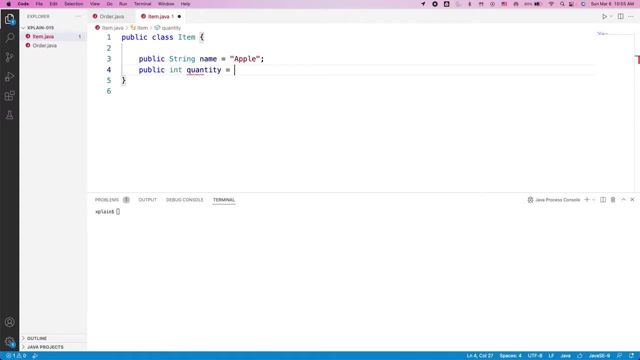 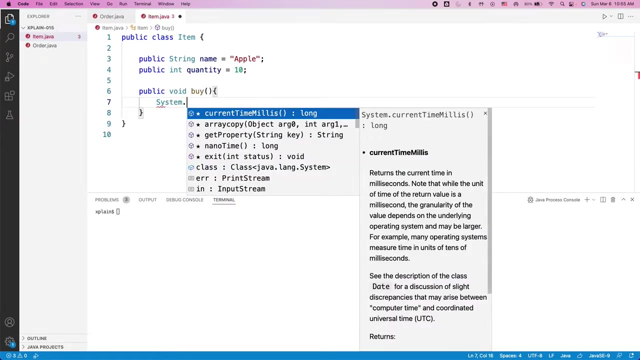 Int Quantity, That's an integer, We'll take that as 10.. And we'll have two methods: Buy and sell Public Void. Buy: This is a method. Within this we will have systemoutprintln And we will say item. 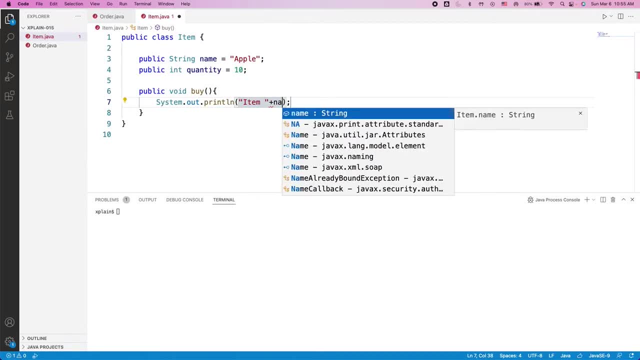 Name of the item With Quantity Quantity Plus. But Similarly We would create A cell method, Void Cell method Within that Vot, With Quantity Call Cell But, And we would do the same for the second method. 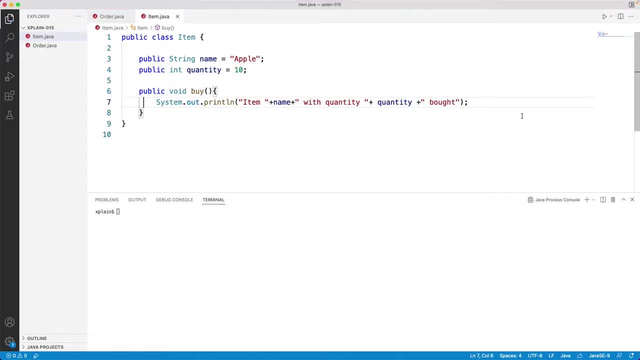 And we would create A cell method, Void Cell method. Within that, The second method: We would create A cell method, A cell method With The Volume, The number of items. Within that we will say systemoutprintln item plus name plus width. 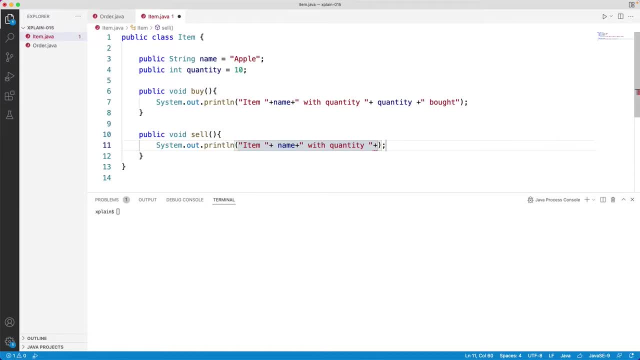 quantity plus quantity plus sold. So we have two methods- buy and sell- which will print the statements as item, with item name and with quantity bought or sold. Now let's go ahead and create a new class called sellItemjava, So within the sellItem we would implement order interface. 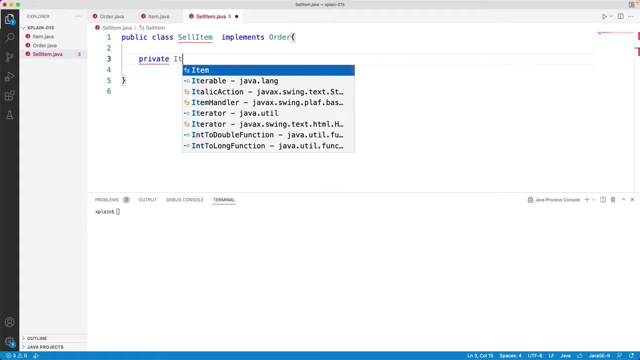 And we will create a new item called appleItem. Within that we will have public sellItem item, appleItem. This is a constructor and we will set this appleItem equals appleItem. So within this we will have the execute method: public void execute. 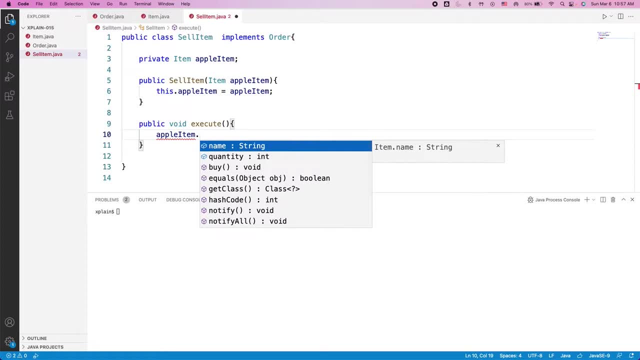 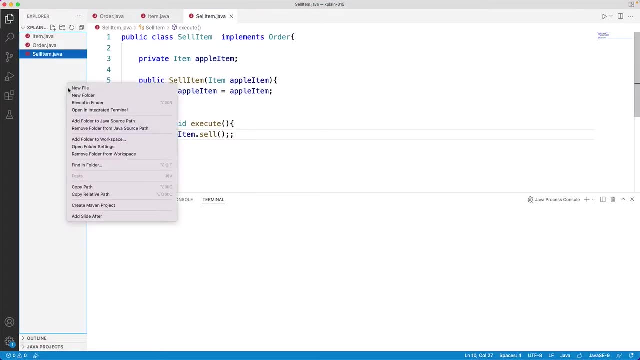 Within this method we will call appleItemsell. We would be selling this item. Similarly, we will create one more class called buyItemjava. That would implement order private item appleItem and create constructor buyItem. The parameters would be item: appleItem. 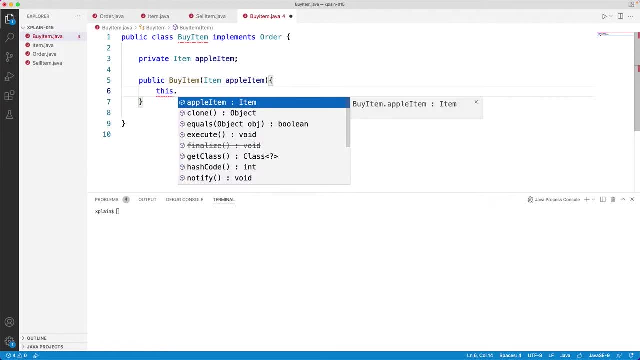